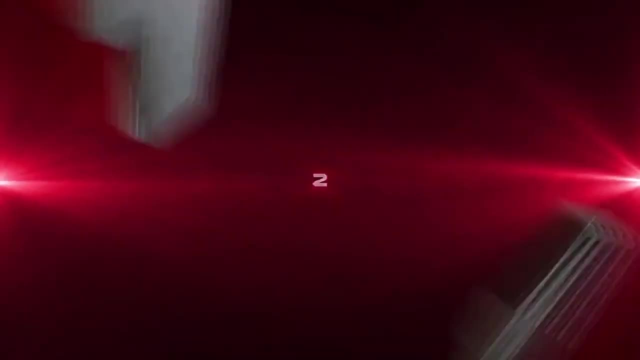 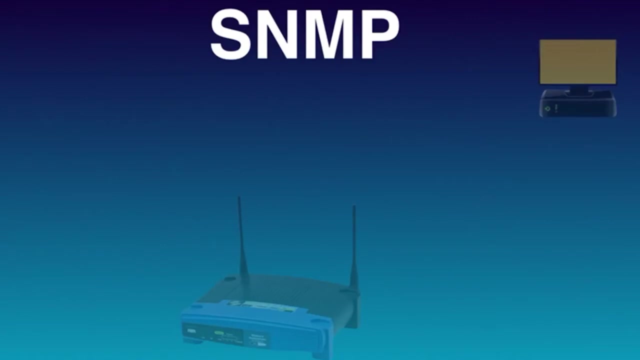 Hello everyone. today in this video, we are going to talk about SNMP. We are going to focus on the absolute basics and I promise I won't get you lost in unnecessary details. Let's get started. SNMP stands for Simple Network Management Protocol. SNMP is an application layer protocol. 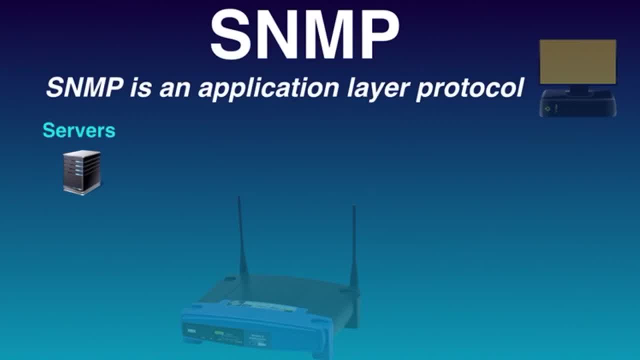 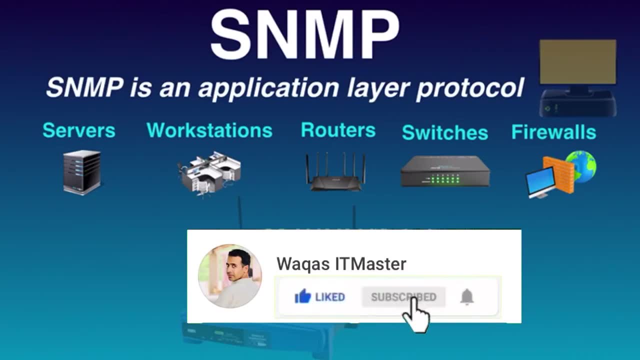 used to manage devices like servers, workstations, routers, switches, firewalls, etc. on an IP network. It's been around since 1980s. Today, it is one of the most widely accepted protocols for network monitoring. SNMP enables the network administrator to monitor network. 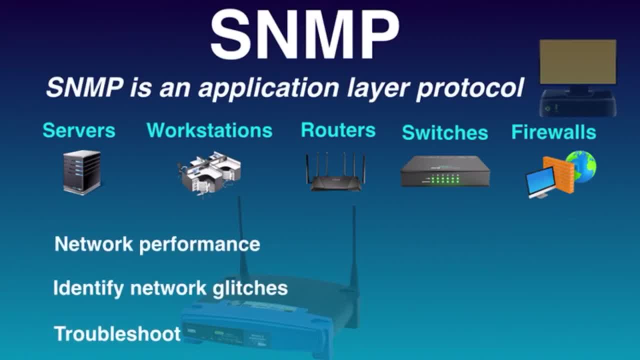 performance, identify network glitches and troubleshoot them. Basically, SNMP is used to control the system, detect network faults and sometimes even used to configure remote devices. Without a protocol like SNMP, there would be no way for network management tools to identify devices, monitor network. 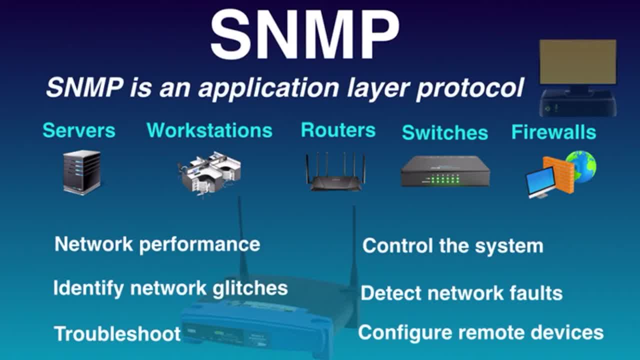 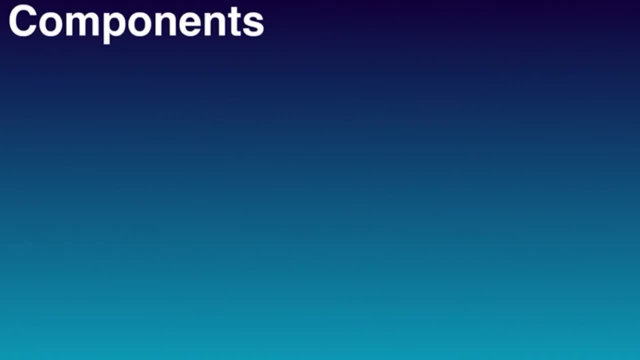 performance, keep track of changes in the network and determine the status of network devices in real time. SNMP is incorporated into three components. First one is SNMP manager. SNMP manager is an application that can be installed on any computer. It is a separate entity that is responsible to communicate with the SNMP agent implemented network devices. 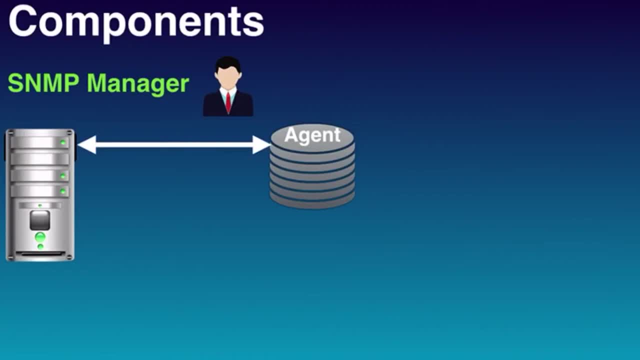 SNMP manager helps Network administrator to manage devices effectively. Functions of managers: Queries agent. gets responses from agents. sets variables in agents. SNMP manager is also known as Network Management System or Network Monitoring System. Second one is Manage devices. A managed device or network element is a part of the network that requires some form of monitoring. 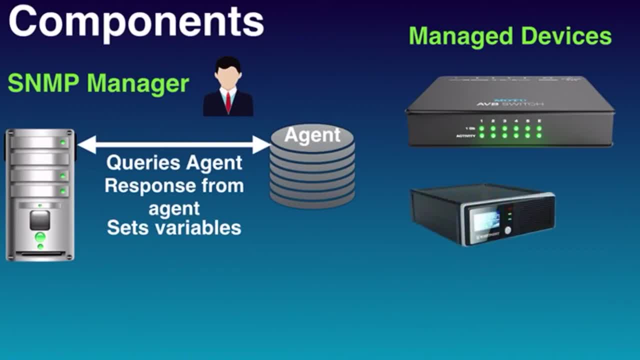 and management, for example, routers, switches, servers, workstation printers, UPS, etc. third one is SNMP agent. agent is a program that is packaged within the network element enabling the agent. allows it to collect the management information database from the device. agent translates the information into a form compatible with SNMP manager. router switch server could be an SNMP agent. 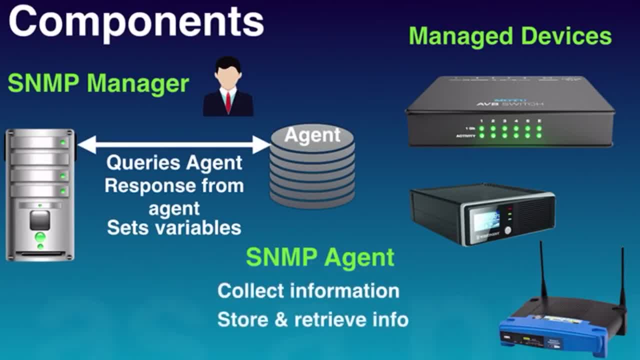 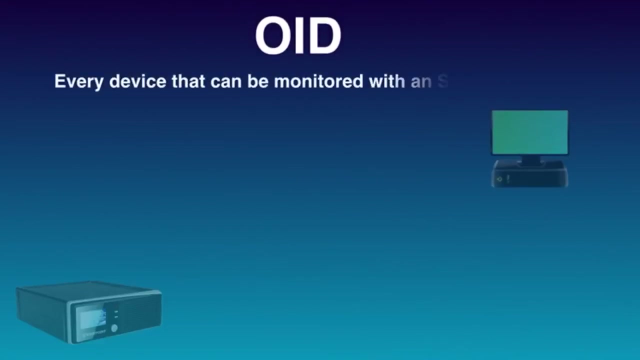 functions of agents. collects management information about its local environment. stores and retrieves management information as defined in the MIB acts as a proxy for some non-SNMP manageable network devices. there are two important terms to remember: OID, MIB- OID stands for object identifier. think of it like this: 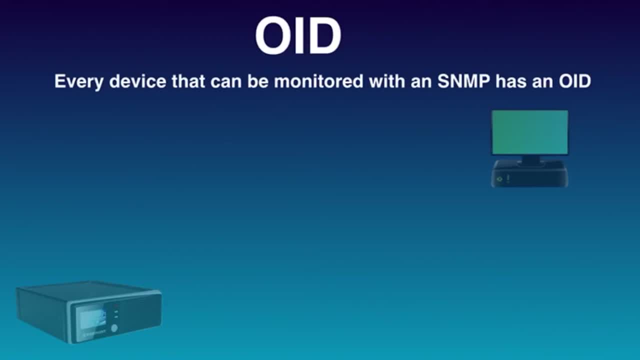 anything and everything on a device that can be monitored: OID, MIB. OID stands for object identifier. think of it like this: anything and everything on a device that can be monitored with snmp has an oid. oid is a numerical number, just like an ip address to identify the device. 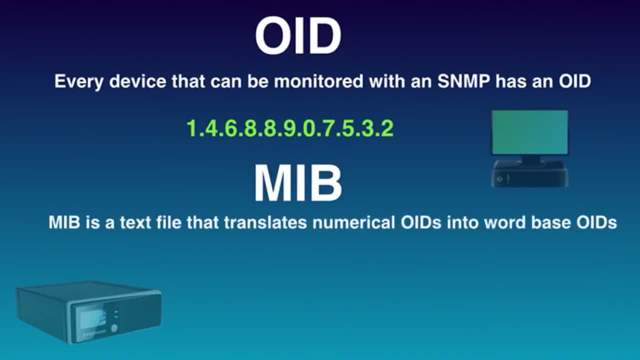 mib stands for management information base. mib is a text file that translates numerical oids into world-based oids. this makes the job of a administrator a lot easier, whatever he is monitoring in the network. let's see how snmp works. snmp talks to the network to find out. 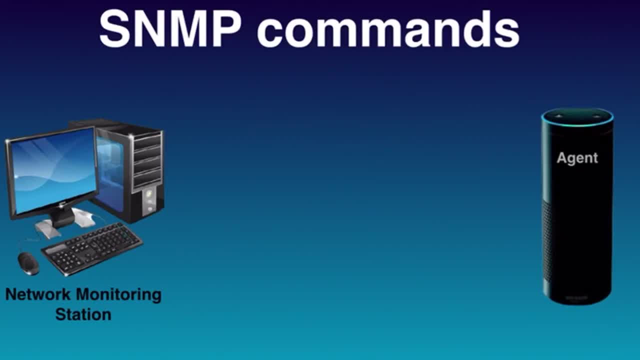 information related to the network device activity, for example bytes, packets, error transmitted and received on a router, connection speed between devices and a number of hits a web server receives. snmp tools perform many functions that rely on a mix of push and pull communications between network devices and 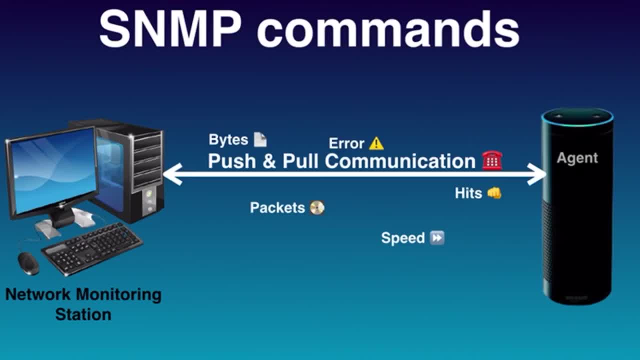 you the network management system. it can execute, read and write commands such as resetting a password or changing a configuration setting. there are two ways to use snmp. first one is polling. second one is notification. polling includes request and response. notification includes traps and informs. get request generated by the snmp manager and sent to an agent to obtain the value. 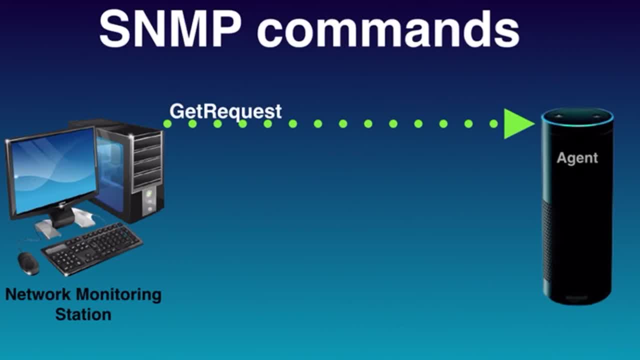 of a variable of the network management system. it can execute, read and write commands such as resetting the sür ней, the RADIR table, classified by its oid response sent by the agent to the snmp manager, issued in reply to a get request. get next request. get bulk. 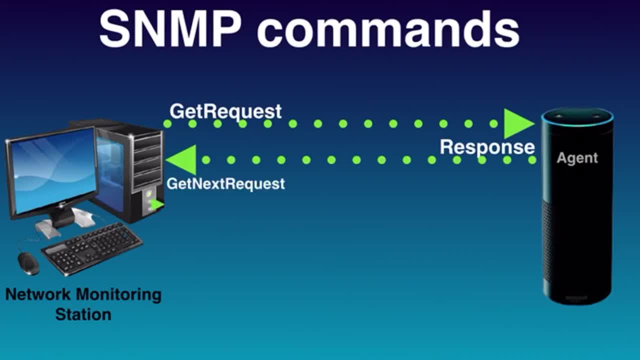 request and a set request. get next request sent by the snmp manager to agent to retrieve the values of the next oid. get bulk request sent by the snmp manager to the agent to efficiently obtain the new will for agencies of Exit and the gets of an expires know 9. recon set defined a cross end response to the agent to the agent to retrieve the value of the next oid. get bulk request sent by the snmp manager to agent to obtain agent to retrieve the values of the next oid. get bulkally request.